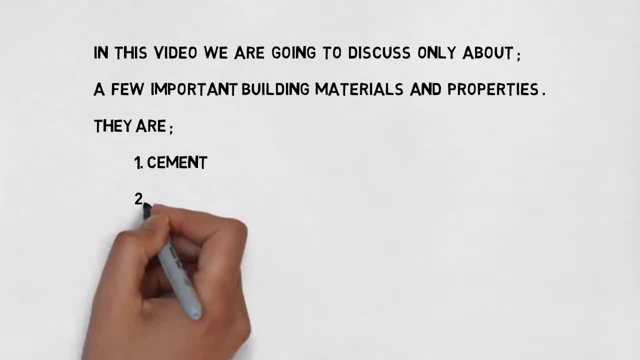 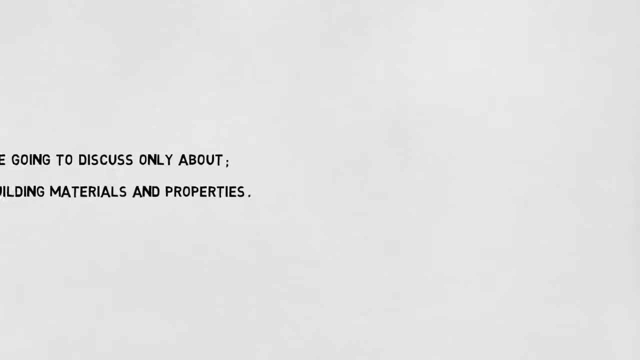 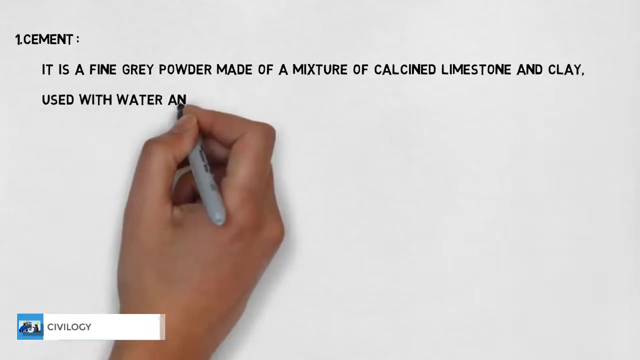 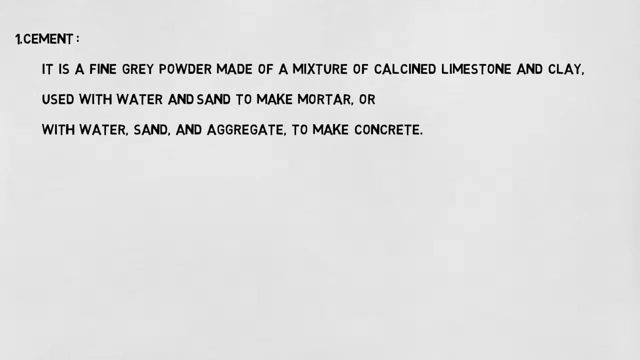 construction. They are cement, steel, sand, concrete and brick. Cement is a very fine gray powder made of a mixture of limestone, limestone and clay used with water and sand to make mortar, or with water, sand and aggregate To make a concrete. basic properties of cement to remember: very smooth and cold when we touch with the head. 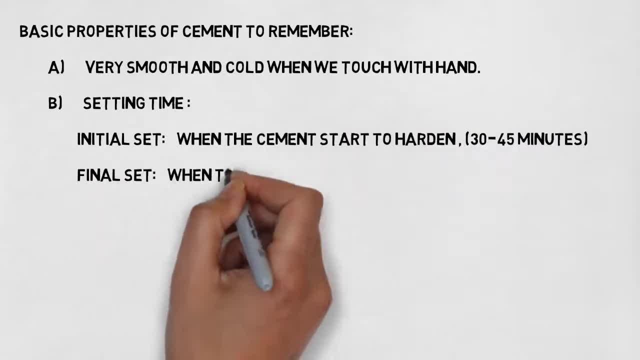 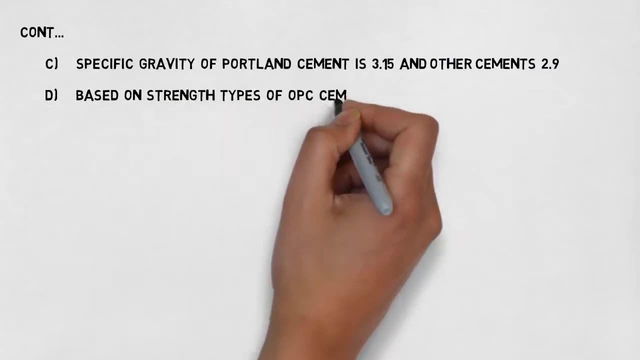 setting time. initial setting time is 30 to 45 minutes, final setting time 10 hours. and it is fine with the wicket upper edges. specific gravity of fortland cement is 3.1- 1.5 and other cements 2.9, based on strength types. 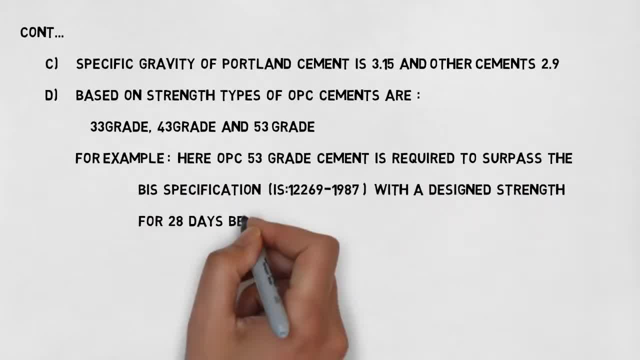 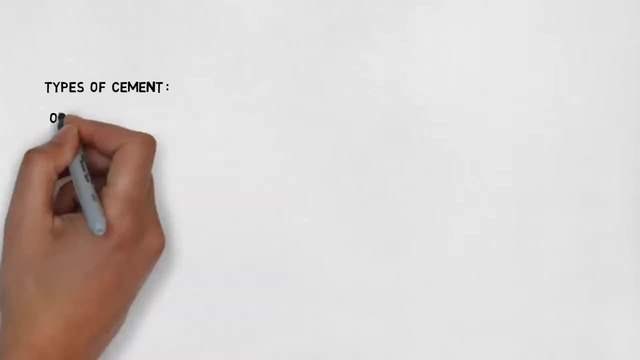 of cements are 33, 43 and 53 grade. here the 53 grade cement means design strength for 28 days for 53 mpa or 530 kg per centimeter square types of cement. and these are the different types of cement. take a screenshot. 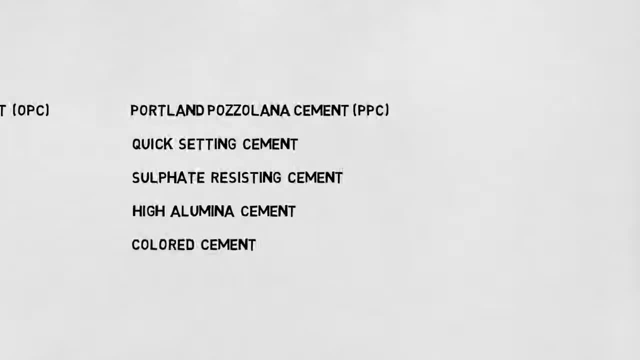 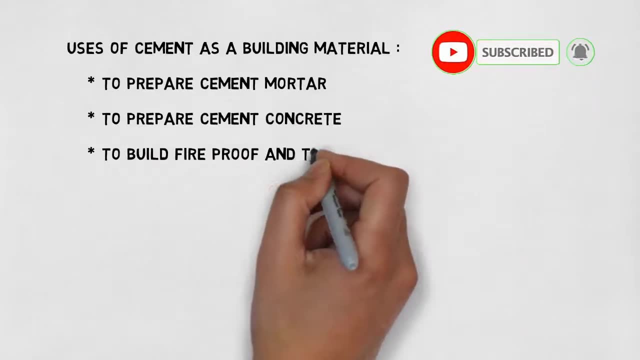 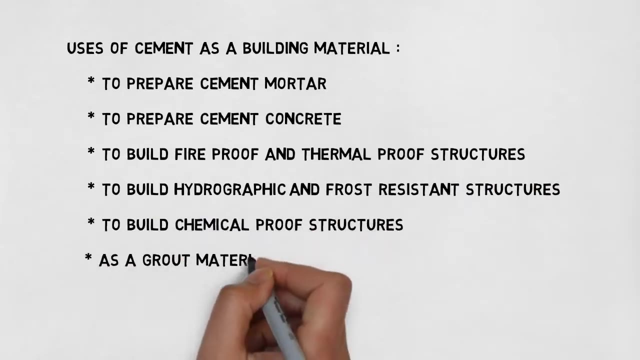 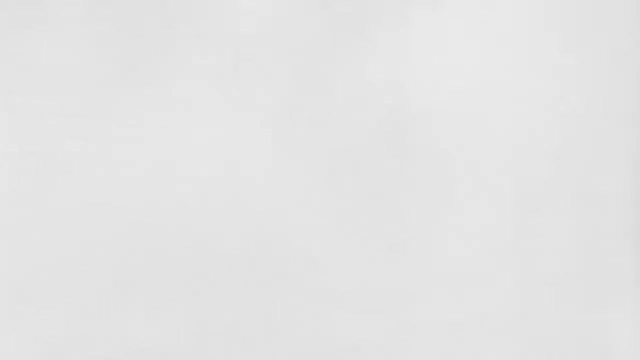 you don't have enough time for discussion. uses of cement as a building material. to prepare cement mortar. to prepare cement concrete. to build fireproof and thermal proof structures. to build hydrographic and frost resistant structures. to build chemical proof structures. also, grout material, steel construction is one of the most important steel using industries. 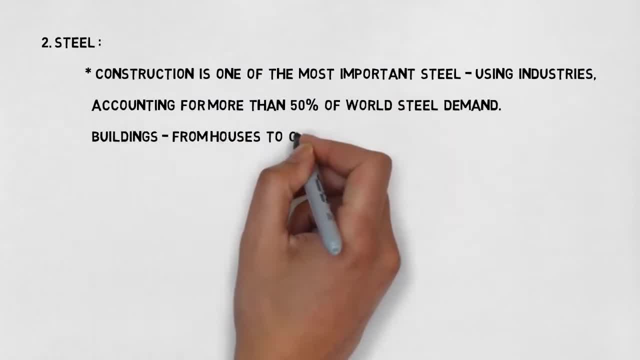 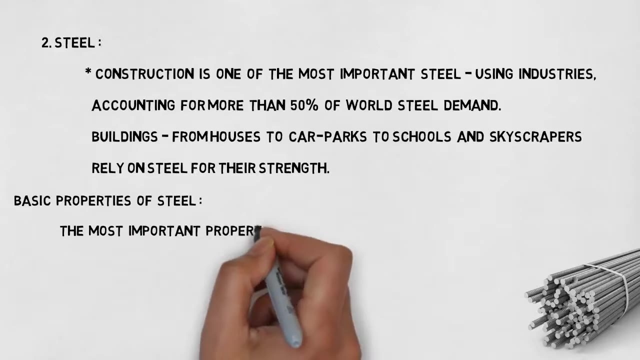 accounting for more than 50 percent of the world steel demand. building, from houses to car parkings, to schools and skyscrapers, rely on strength of steel. basic properties of steel. the most important properties of steel are great formability and durability, good tensile yield strength and good thermal conductivity. types of steel used in construction or structural steel: 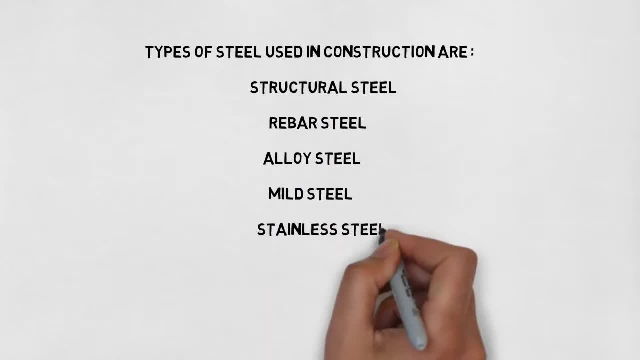 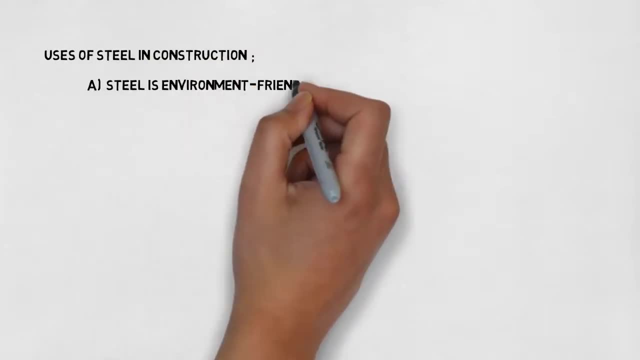 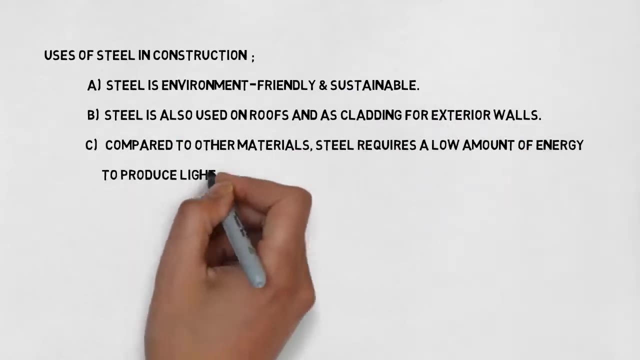 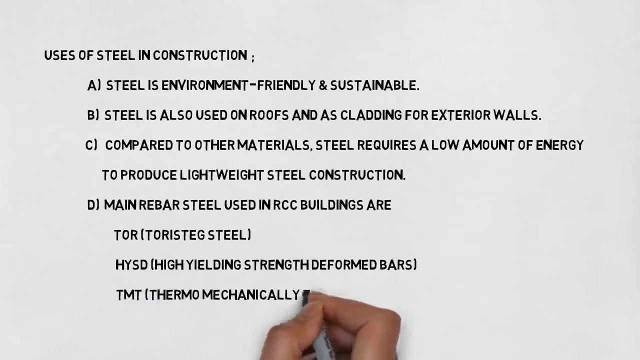 rebar alloy. mild stainless tool, light gauge steel. use of steel in construction. steel is environmentally friendly. steel is also used in roofs. compared to other materials, steel requires a low amount of energy to produce lightweight steel construction may rebar steel used in construction or tor, hysd, tmd. 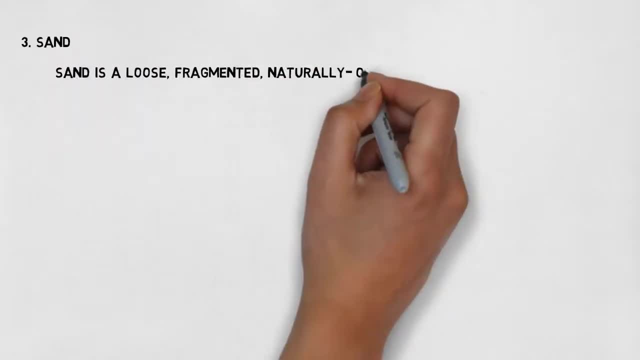 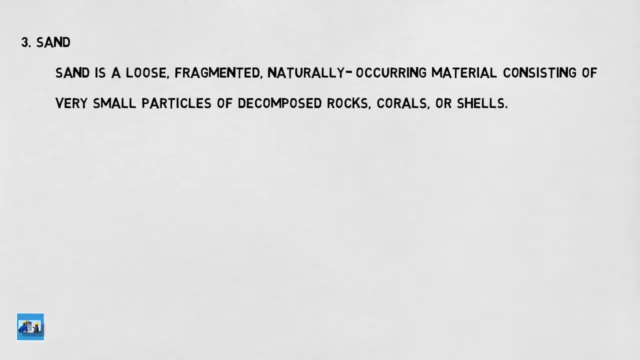 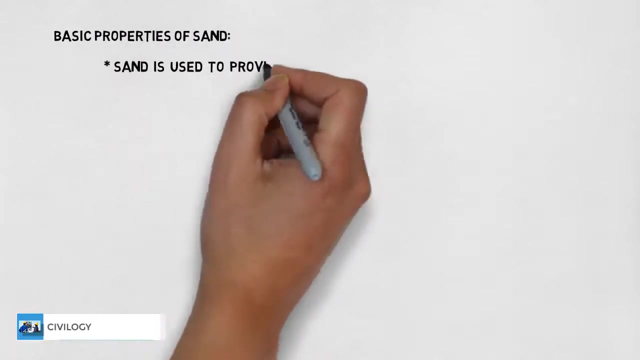 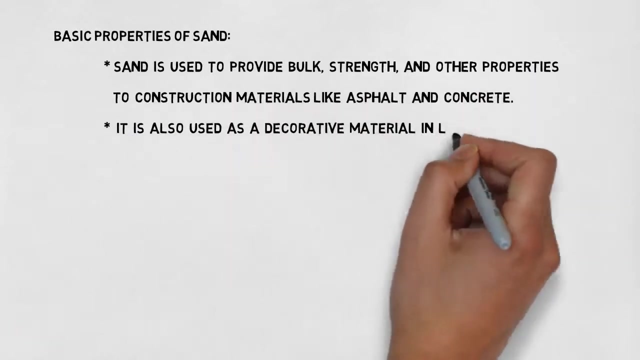 sand. sand is a loose, fragmented, naturally occurring material consisting of various small particles of decomposed rocks, corals or shells. basic properties of sand sand is used to provide bulk. strength and other properties to construction materials like asphalt and concrete. it is also used as decorative material in 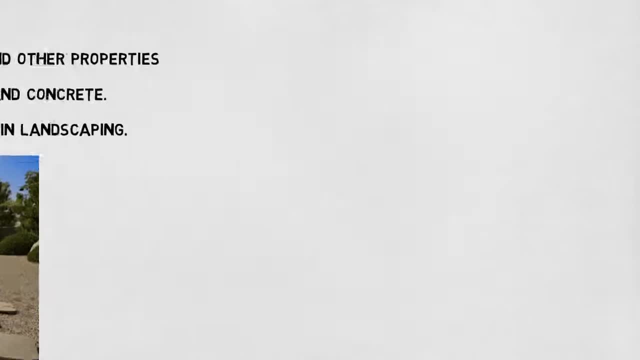 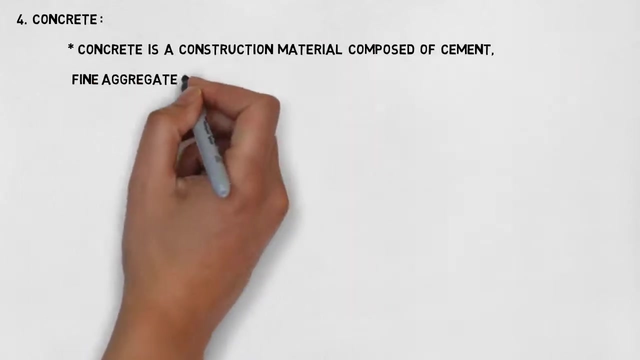 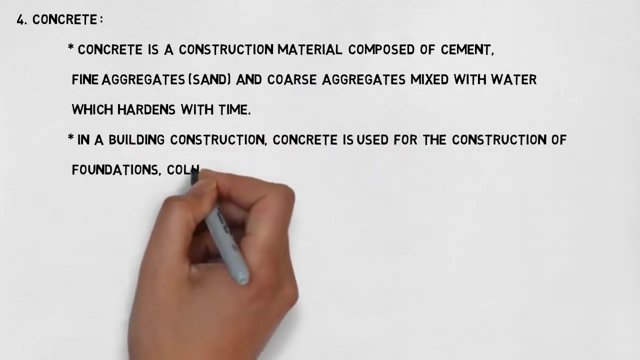 landscaping. types of sand: concrete sand crushed stone, utility sand, fill sand, weed sand. concrete concrete is a construction material composed of cement, fine aggregates and coarse aggregates mixed with water, which hardens with time in a building material. construction concrete is used for construction of foundations, columns, beams, slabs and other load bearing. 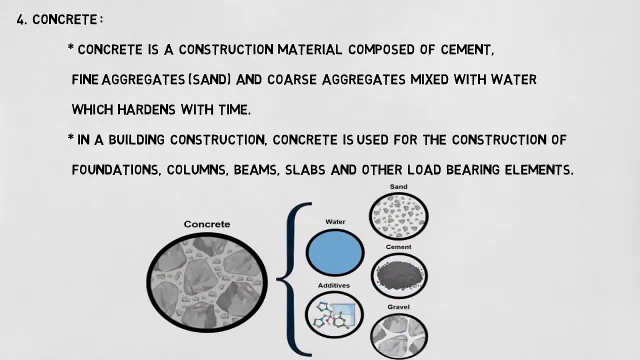 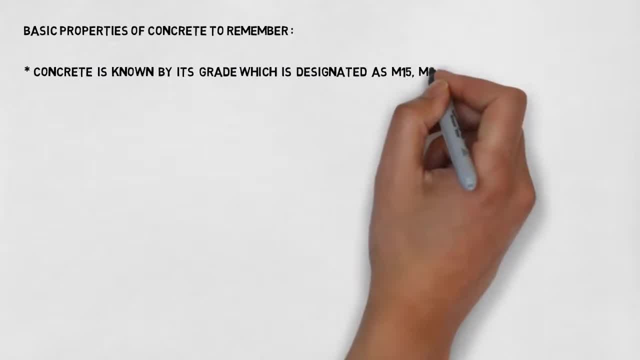 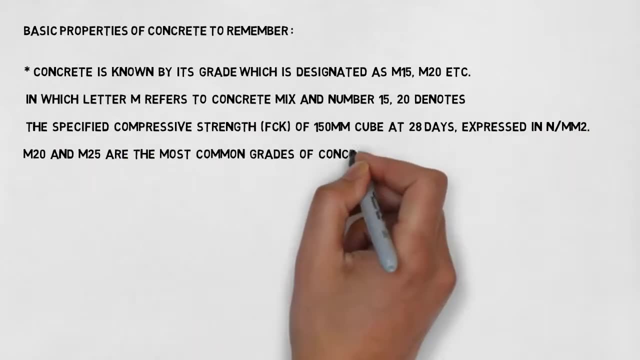 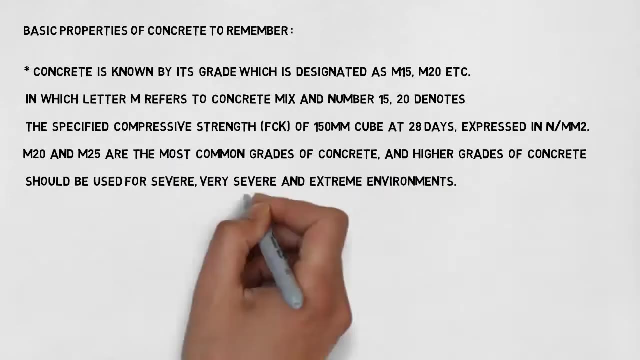 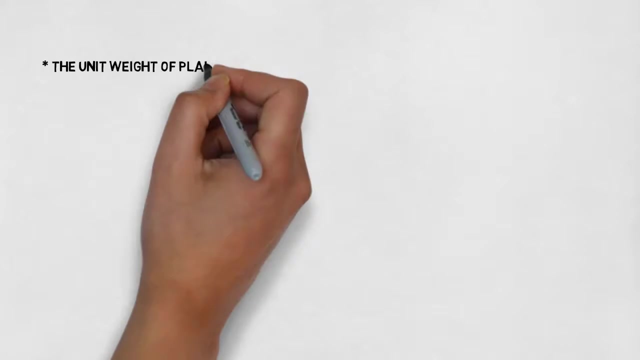 elements: basic properties of concrete. to remember, concrete is known by its grade, which is designated as m15, m20 and etc. which M prefers here mix, and number denotes its compressive strength in Newton per mm square. the unit weight of plain and reinforced concrete as specified by is 456 for 24. 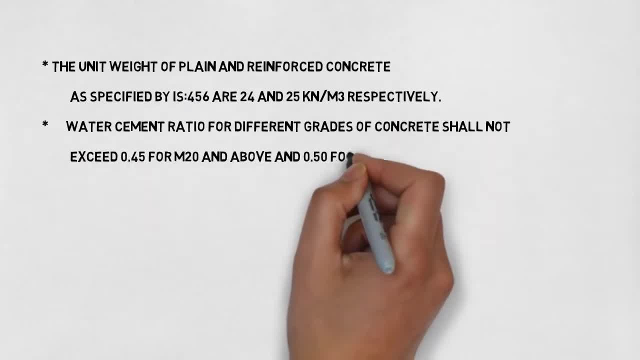 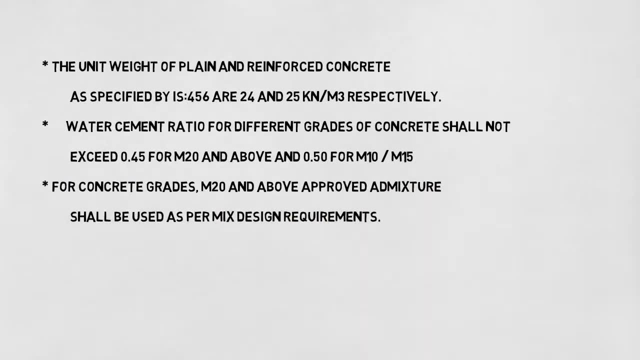 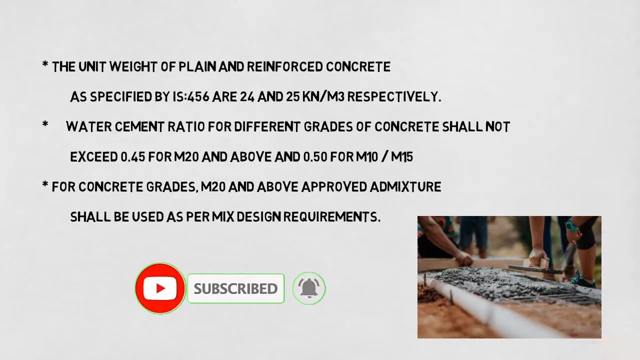 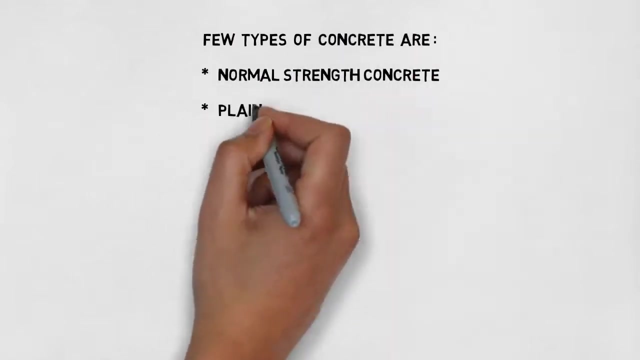 and 25 kilo newton per meter cube. water cement ratio for different grades of concrete shall not exceed 0.45 for M20 and level and 0.5 for a mountain and a fiction. few types of concrete or normal strength concrete, plain or ordinary concrete.